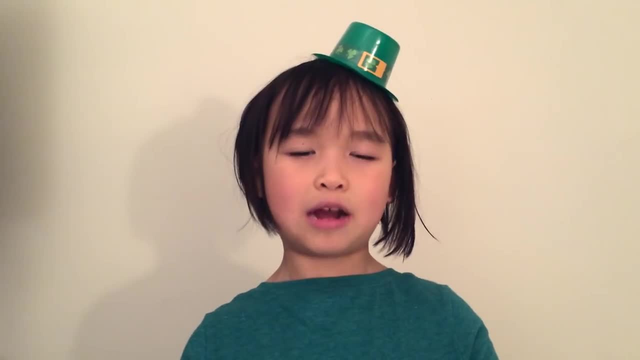 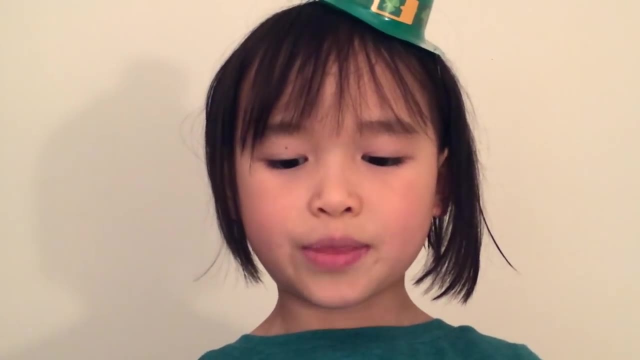 And this one is the other one, And they're both about a leprechaun. There once was a little green man who went to the farm for a lamb. On the way he found something on the ground and he got butted by a ram. 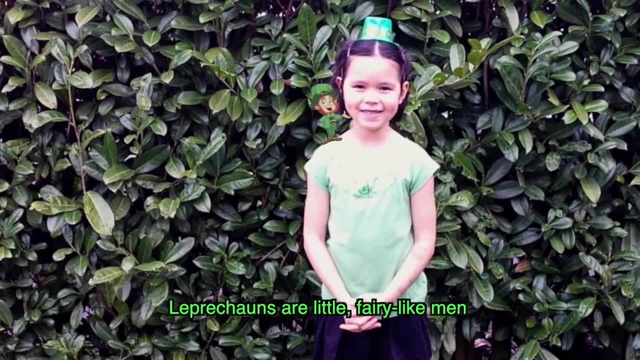 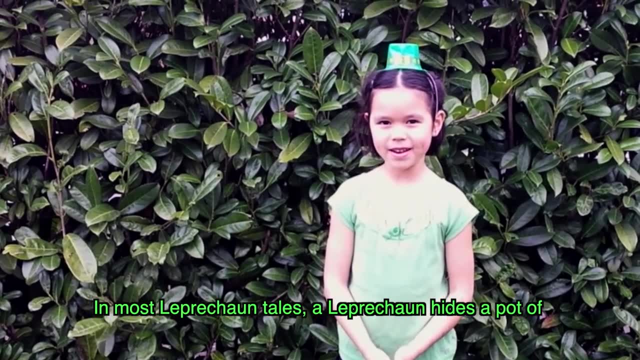 Today we're going to talk about leprechauns. Leprechauns are little fairy-like men who are often cobblers. In most leprechaun tales, a leprechaun hides a pot of gold at the end of a rainbow. 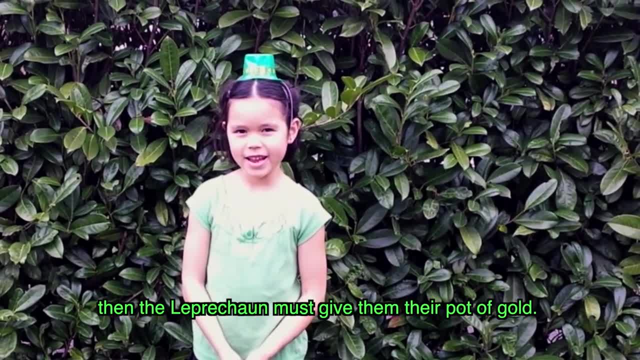 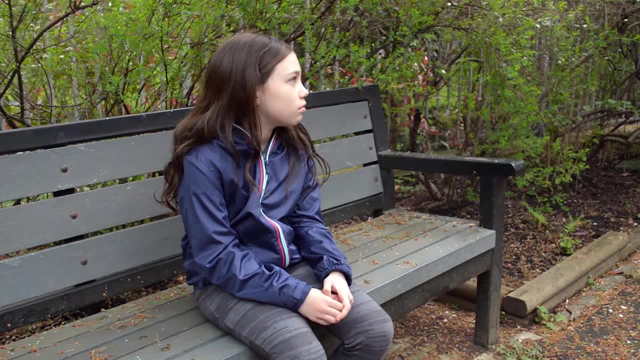 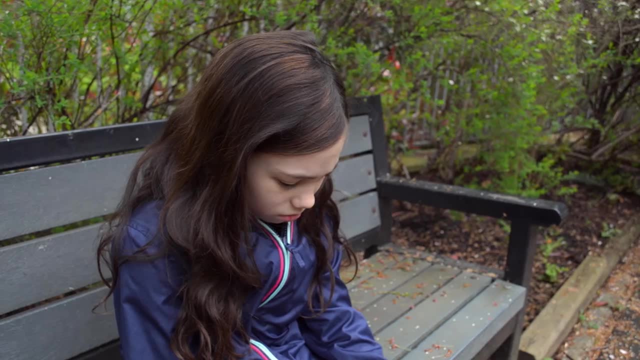 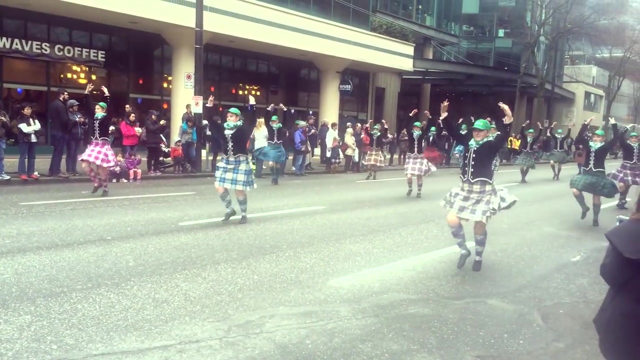 If a person catches them, then the leprechaun must give up the pot of gold. I remember when I went to the Irish parade. While we were there, we saw some Scottish dancers. We also saw flute players and a marching bagpipe band. 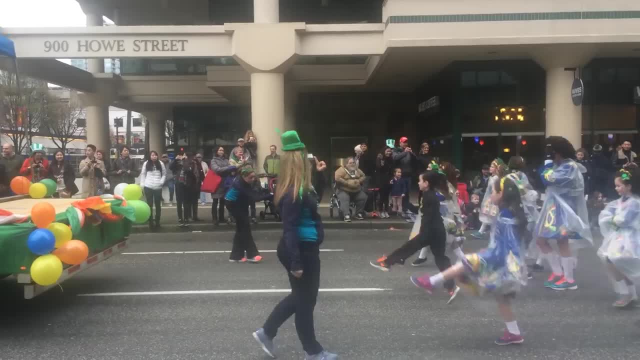 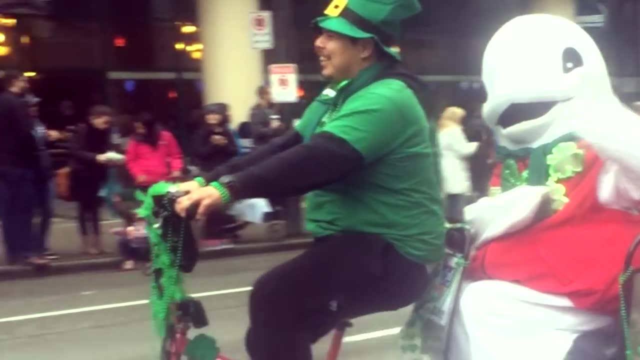 And we also saw some Irish dancers on a parade float. Hey look, that's me. We got some pins and balloons- Look at that happy little face- And a leprechaun on a bike with a bloke oil. Oh, and fiddlers. 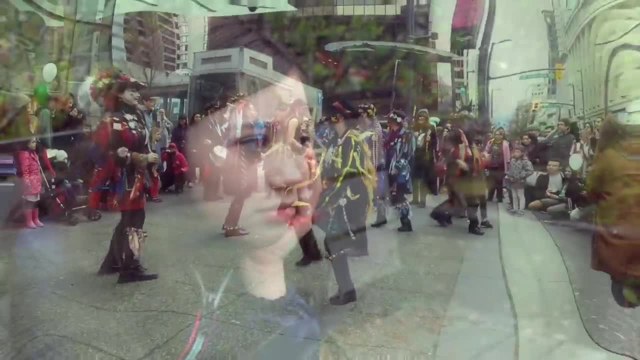 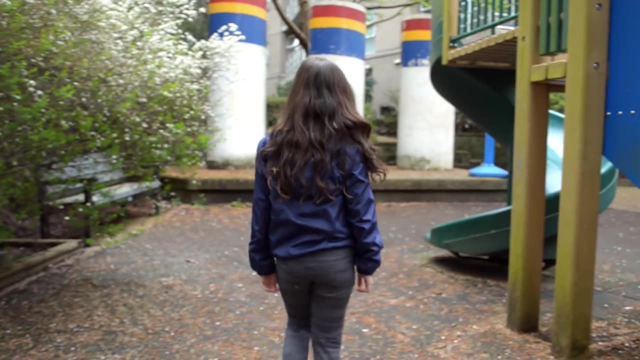 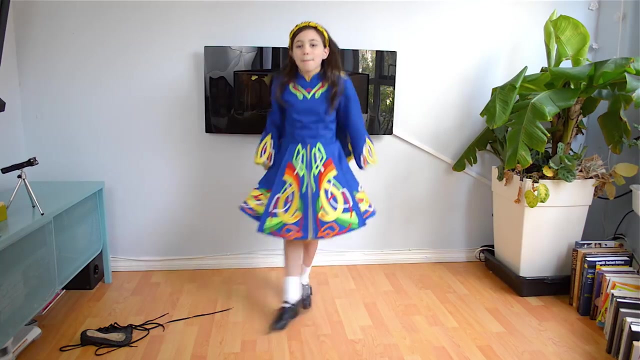 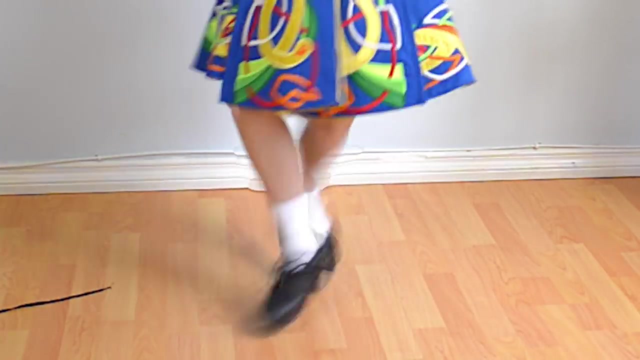 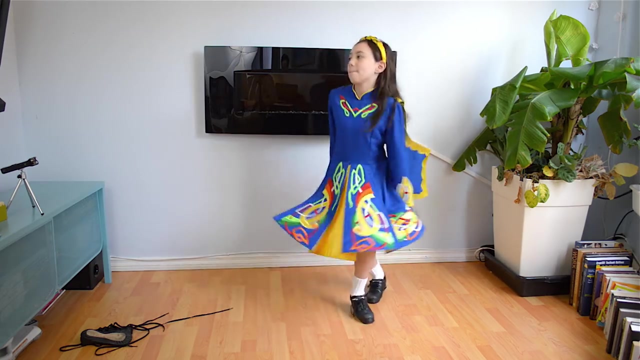 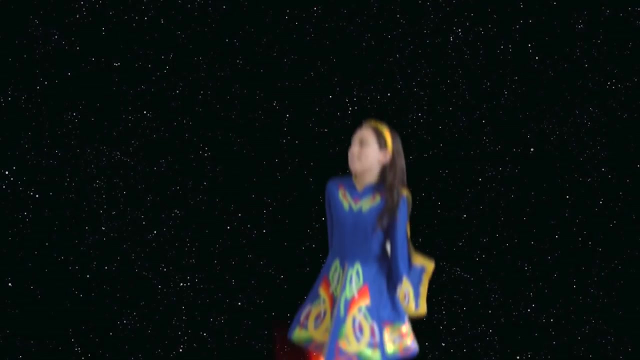 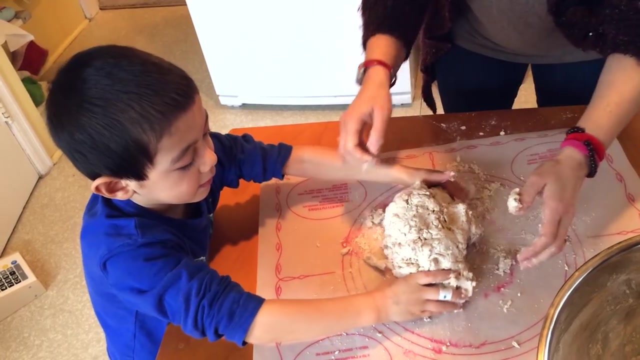 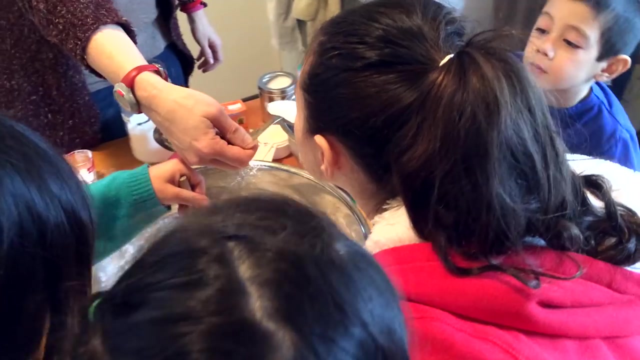 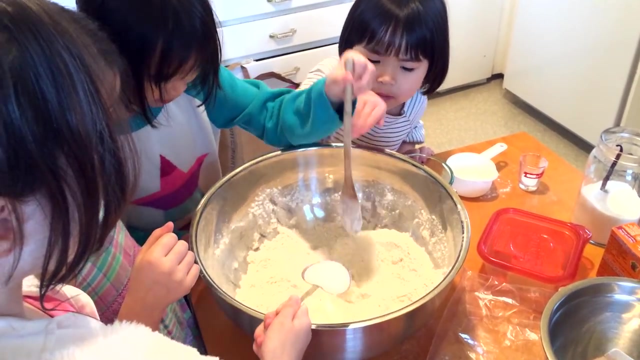 and Moorish dancers. Oh yeah, good times. Now I'm going to show you a full dance called Treble Reel. Now I'm going to show you a full dance called Treble Reel. Let's go. Today, we learned about leprechauns. 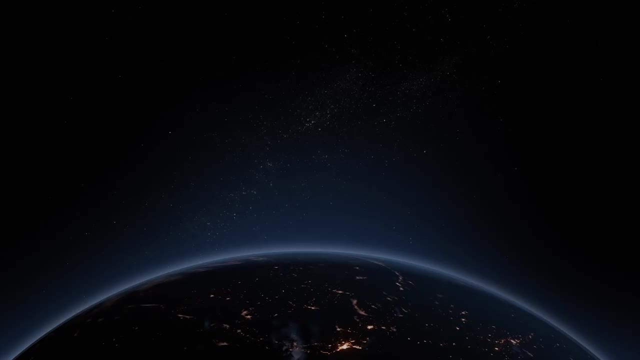 heard some Irish fiddle music and watched some Irish dancing. We're going to watch another one, but we're going to watch something else too, So don't forget to subscribe to our YouTube channel and hit the bell, And we'll see you in the next one. 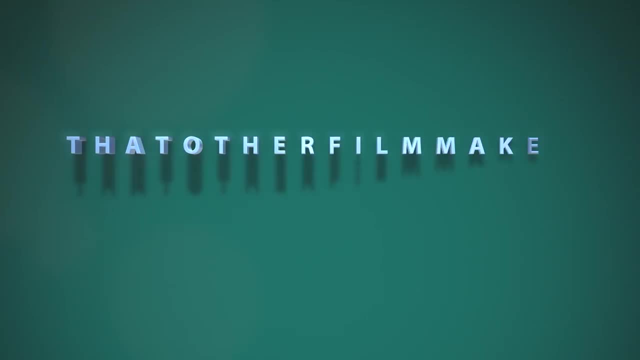